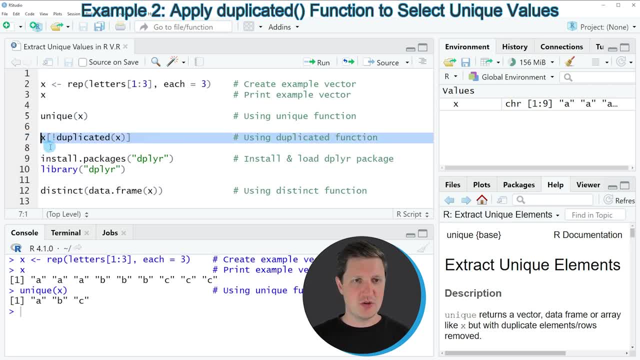 And you can see that example in line 7 of the code. So in this line of code I'm specifying the name of our data object And then I'm subsetting this data object using square brackets, and within the square brackets I'm using the duplicated function to check which elements of our data object are not duplicated. 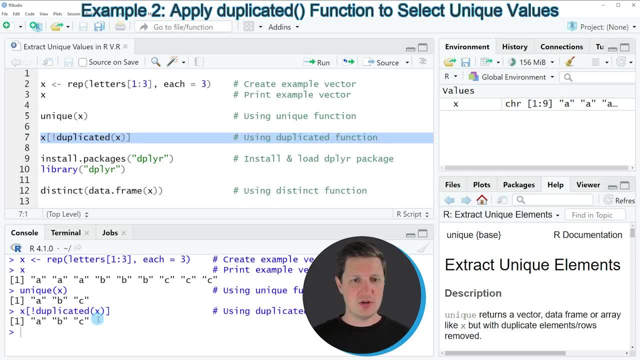 So if you run line 7 of the code, you can see that our output is returned again. So the output of line 7 is exactly the same as the output of line 5.. However, this time we have used the duplicated function to return unique values from our data object. 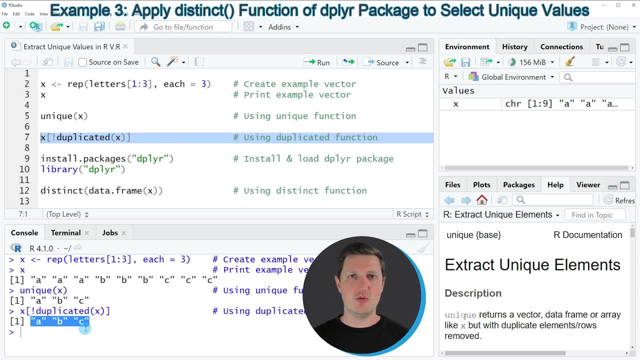 In the next example, I want to show you that it is also possible to use the deep layer package to extract unique values from a data object. So in order to use the functions of the deep layer package, we first need to install a new function. 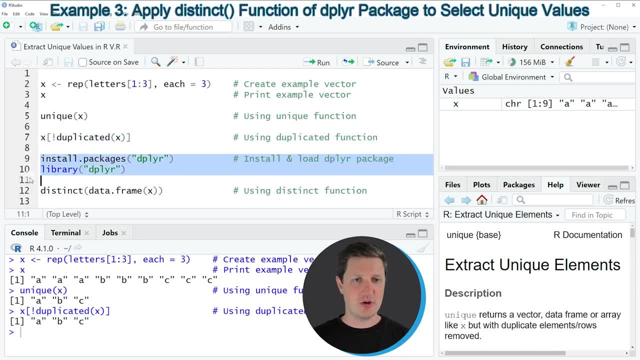 load the dplyr package. as you can see in lines 9 and 10 of the code, I have installed the dplyr package already, so for that reason I'm just going to load it, as you can see in line 10, and after running this line of code we are able to: 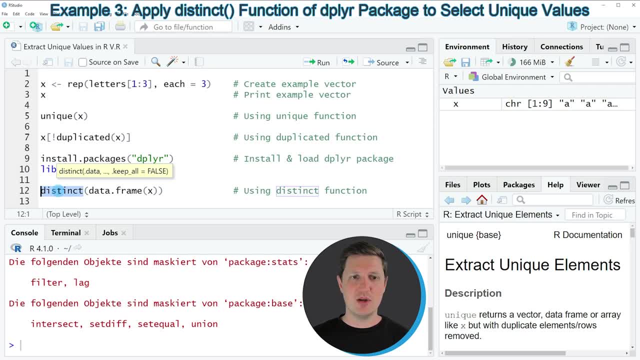 use the distinct function that is provided by the dplyr package, as you can see in line 12.. So if we want to use the distinct function, we can apply the code that you can see in line 12, and in this line I'm applying the distinct function. 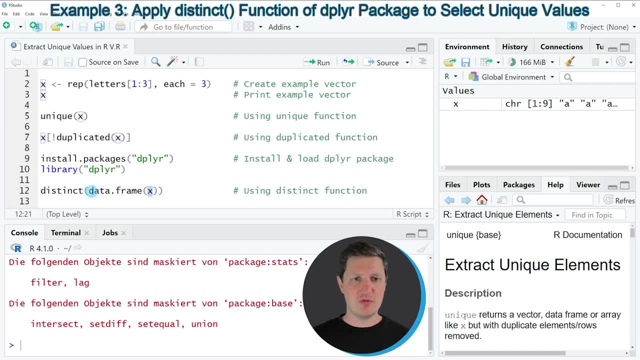 to our data object. however, before I can apply the distinct function, I also need to convert our vector object to the data frame class. So if you run line 12 of the code, you can see that another output is created and, as you can see, this output. 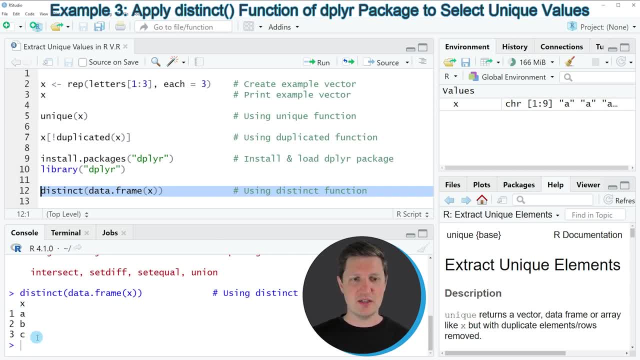 is a data frame. however, the rows of this data frame show the unique values in our data object x. So in this tutorial, I have explained how to extract unique values from a data object using the R programming language. However, in case you want to learn more on this topic, you could check out my home page. 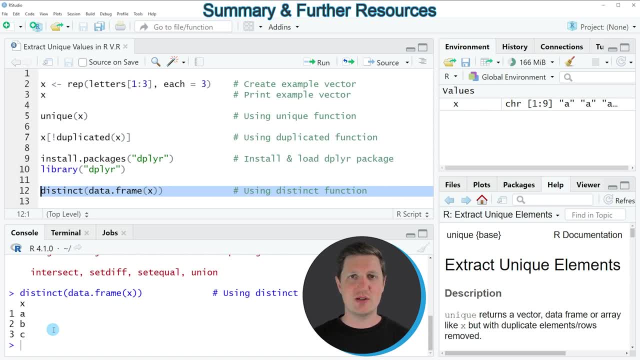 statisticsglobecom, because on my home page, I have recently published a tutorial in which I'm explaining the R programming code that I have shown in this video in some more detail, and I will put a link to this tutorial into the description of the video. Furthermore, if you have liked the video, I would be.